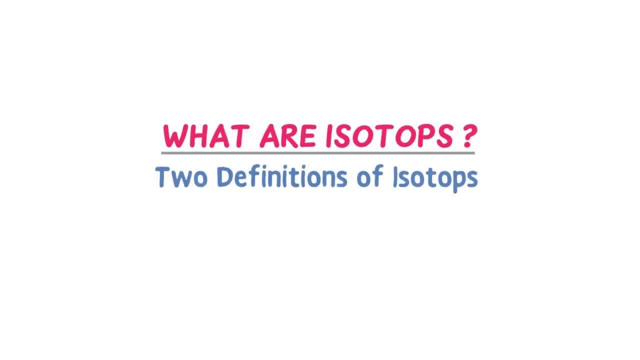 What are isotopes? Two different and unique definitions of isotopes. Before starting the lecture, click on the subscribe button and get access to our hundred of conceptual lectures for free. Well, we know all about atomic structure. An atom is made up of three tiny particles. 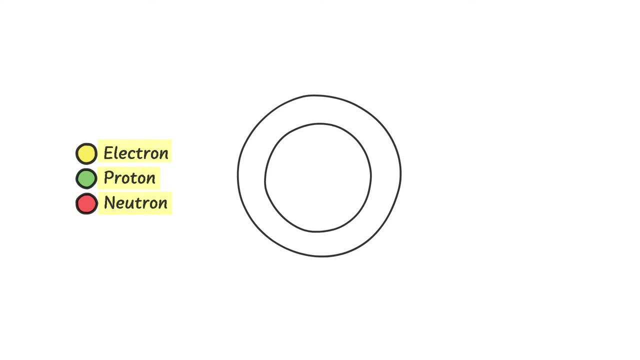 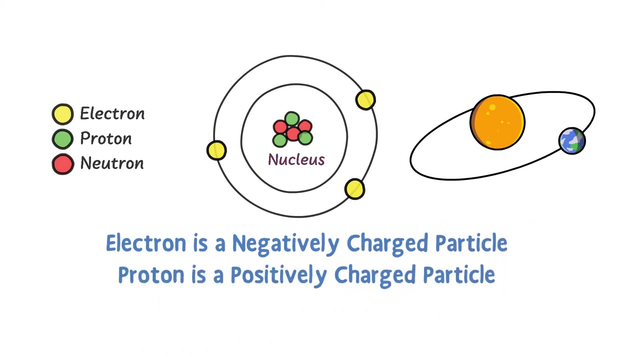 like proton, neutron and electron. Protons and neutrons live in the nucleus, while electrons revolve around the nucleus In these fixed parts are shells, just like planets revolve around the sun. Remember that electron is a negatively charged particle and proton is a positively charged. 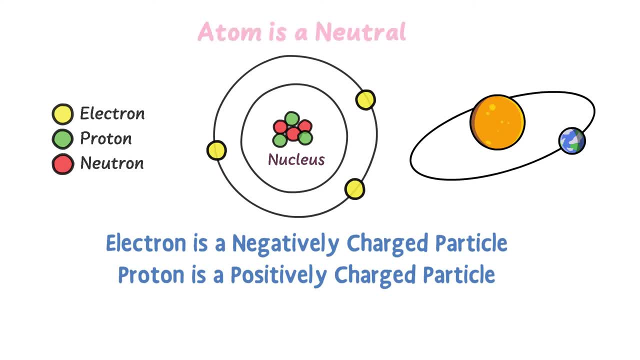 particle, An atom as a whole, is electrically neutral Because the number of protons is equal to the number of electrons inside any atom. Let me repeat it: The number of protons is equal to the number of electrons inside any atom. Now, what are isotopes? 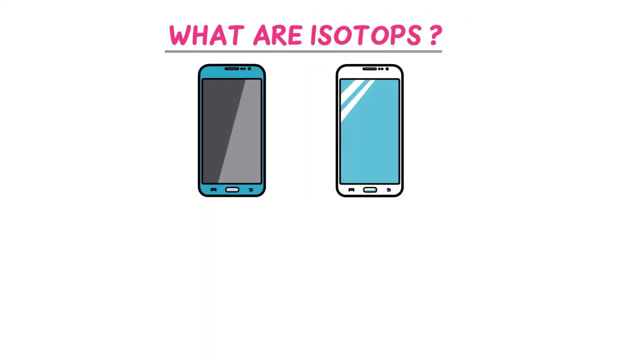 Let consider these cell phones, Let they both are launched by the same company. They have the same functions, same shapes and same properties, But there is only one difference between them. I mean difference in color: One is white and the other is blue. 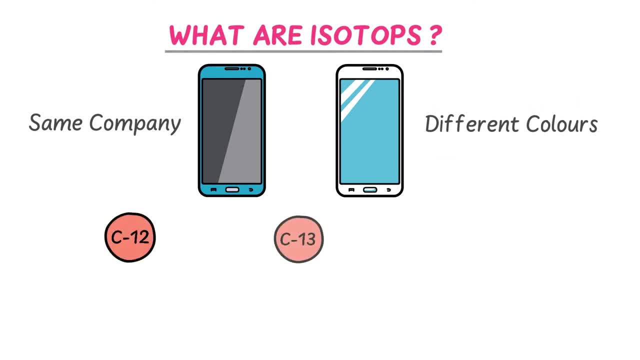 Now consider carbon 12,, carbon 13 and carbon 14.. As these cell phones are from the same company, similarly these atoms are from the same element. Also, there is only difference in color between these cell phones, So here there is only. 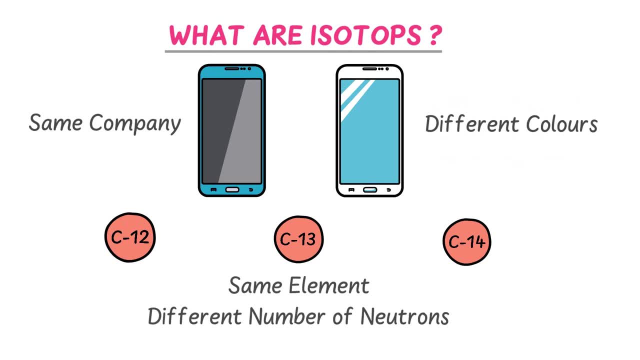 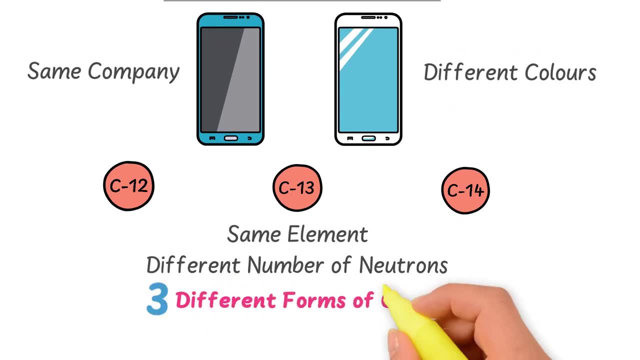 There is only difference in number of neutrons among these atoms. Carbon 12,, carbon 13 and carbon 14 are three different forms of the carbon element. In carbon 12, there are six protons, six electrons and six neutrons. 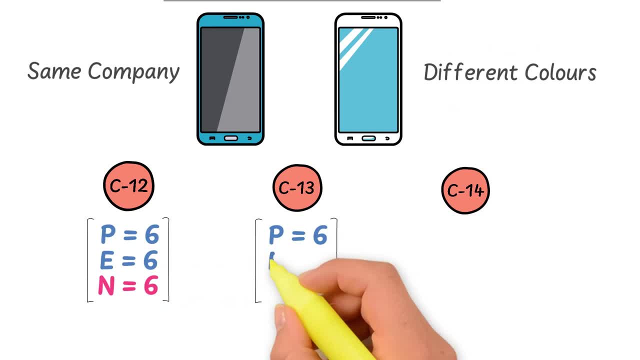 In carbon 13, there are six protons, six electrons and seven neutrons, While in carbon 14, there are six protons, six electrons and eight neutrons. From this example, you can learn that all these carbon atoms have same number of protons and electrons. 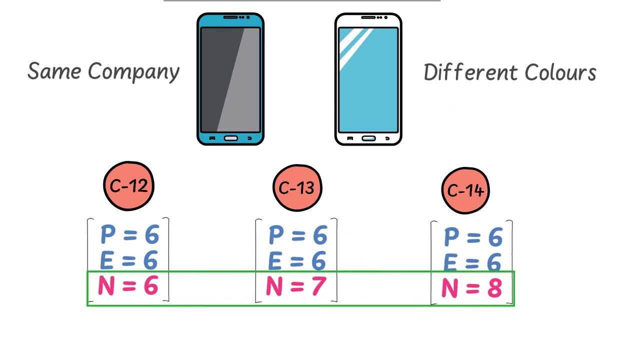 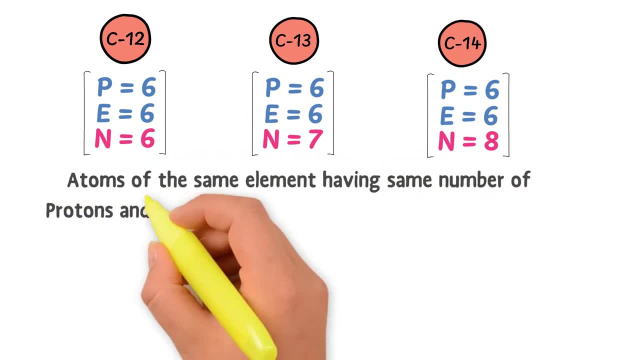 but they have different number of neutrons. So we therefore define isotopes as atoms of the same element having same number of protons and electrons, but different number of neutrons. Let me repeat it: Atoms of the same element having same number of protons and electrons. 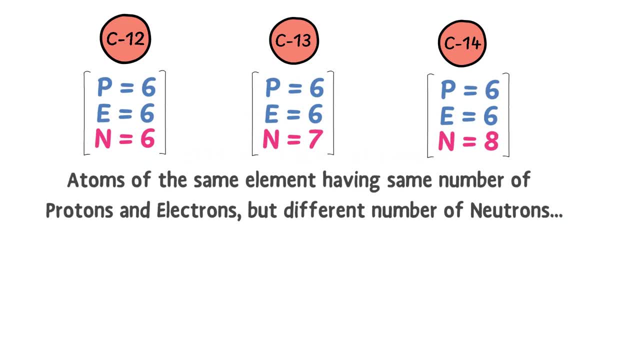 but different number of neutrons. Note it down, this important point, that isotopes have same chemical properties because they have same number of electrons and outermost shell. Secondly, isotopes have different physical properties because they have different number of neutrons and the nucleus. 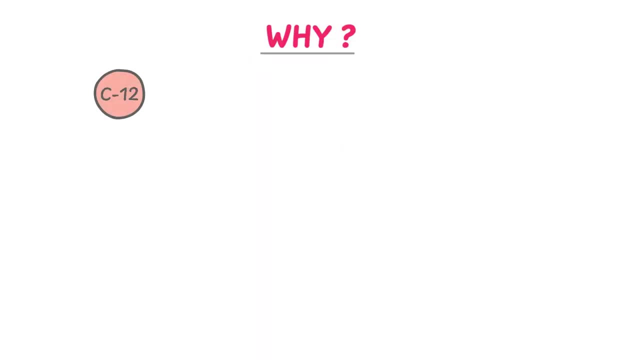 Now why we call these atoms neutrons and neutrons neutrons. Why we call these carbon atoms as carbon 12,, carbon 13 and carbon 14?? Well, it is because of their respective masses. For example, in carbon 12, there are six protons and six neutrons. 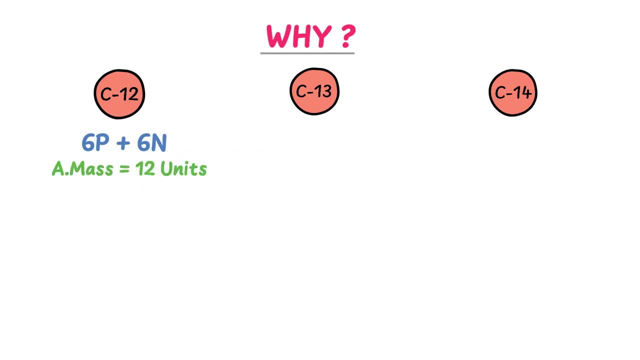 So its atomic mass is 12 units and its atomic number is six units because of six protons. So we therefore call it carbon 12.. Also, in carbon 13, there are six protons and seven neutrons. So its atomic mass is 13 units and its atomic number is again six units because of six protons. 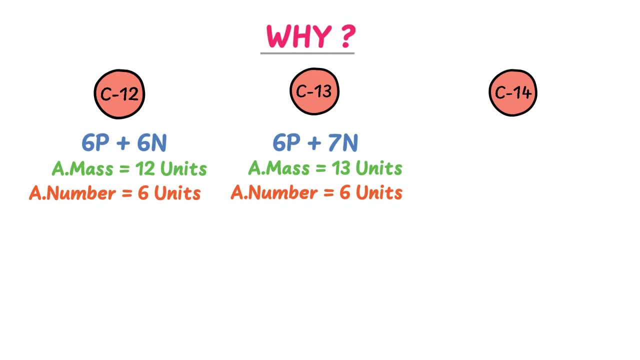 So we call it carbon 13.. Similarly, in carbon 14, there are six protons and eight neutrons, and its atomic mass is 14 units and its atomic number is again six because of six protons. So we therefore call it carbon 14.. 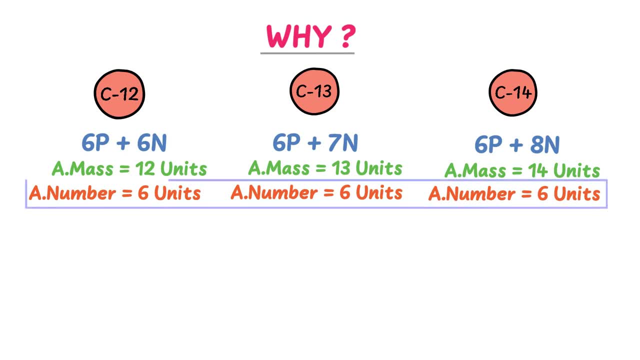 Hence we call it carbon 14.. Now look at the atomic numbers of these atoms. They all have same atomic numbers. I mean six units, because they all have six protons. but they have different atomic masses because of having different number of neutrons.